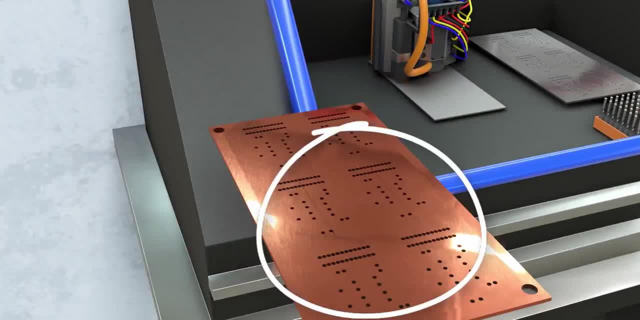 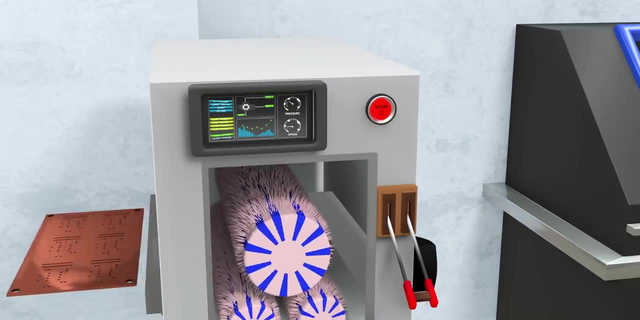 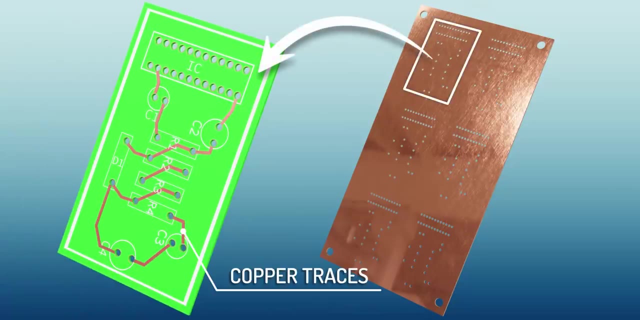 These holes are used to attach the components into the board. later on, After drilling, the boards are cleaned properly so that no drilling residue is left behind. Now the most important step: production of these tiny and complex copper traces. The best way to achieve this is by a chemical process called etching. 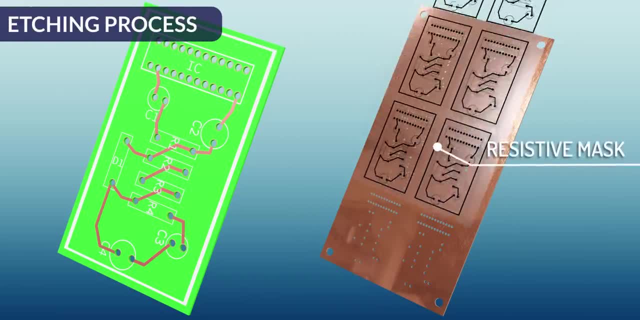 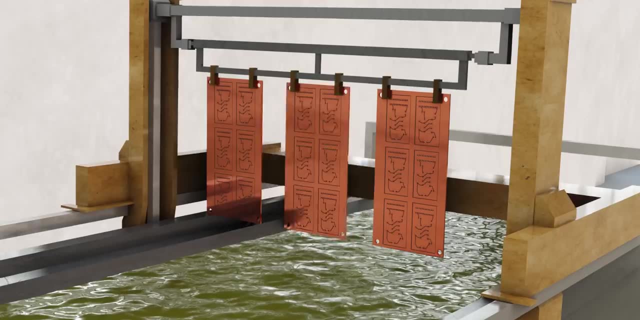 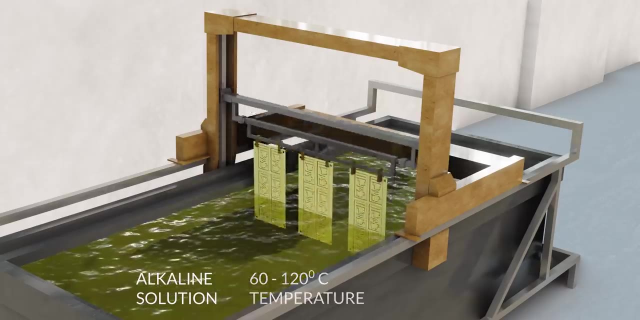 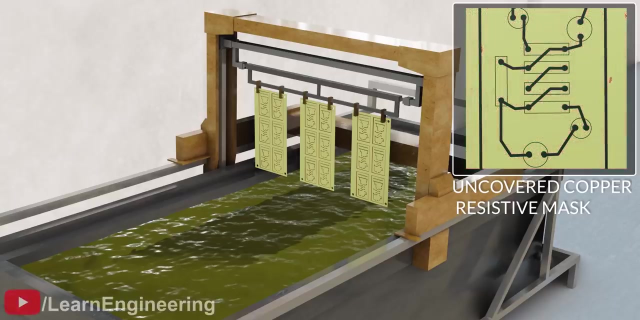 where you have to cover the copper plate with a resistive mask. This resistive mask will have the same pattern of the circuit you want. Now, if you dip this arrangement into an alkaline solution at 60 to 120 degrees Celsius, the area of copper uncovered by the resistive mask dissolves or is etched away. After this process is 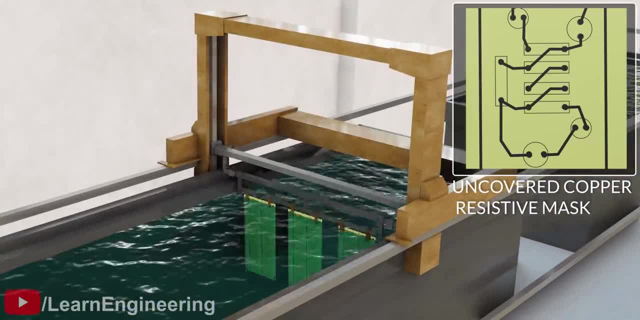 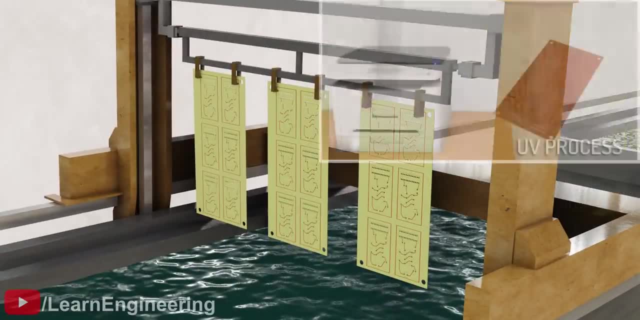 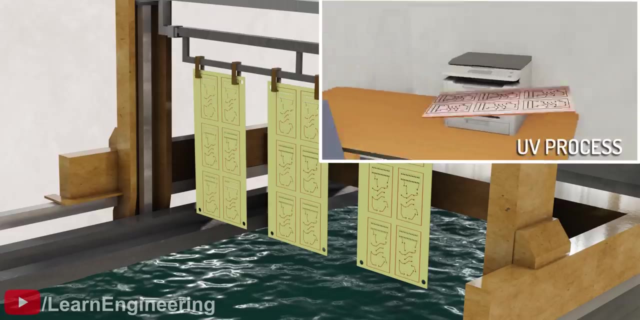 complete, the protective mask is washed off as well. Thus, we are left with only required traces of copper. The circuit prints on the resistive mask used in this process is obviously made with the help of a Gerber file. A UV-light-based technique is used for sticking the mask to the copper plate where it is needed. 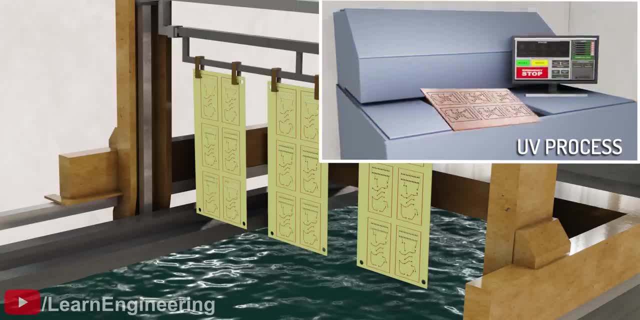 To achieve bulk manufacturing, multiple masks are made in a single sheet, As you can see, we can also use a UV light to light the top of the circuit. As you can see, we also don't need to do this. It's only a matter of adding more materials. 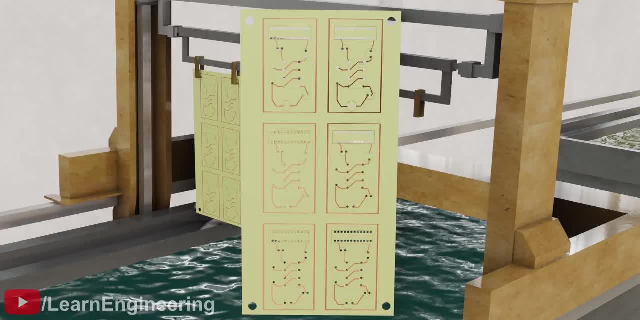 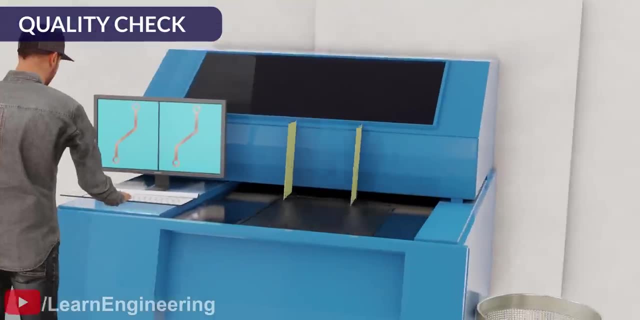 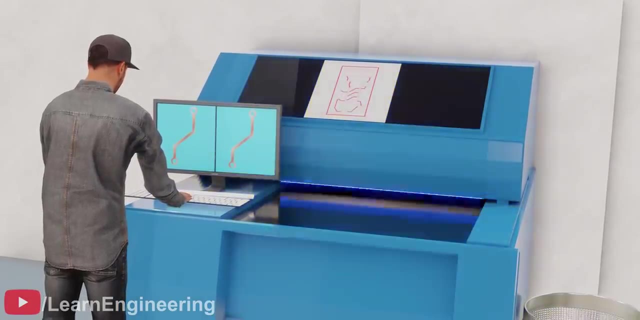 As you can see, the copper traces are very thin, hardly visible to the naked eye. To check the quality of the copper traces, the boards go for an inspection. An operator with an optical inspection machine checks the quality of printed boards by taking pictures of them and comparing them with the design files. 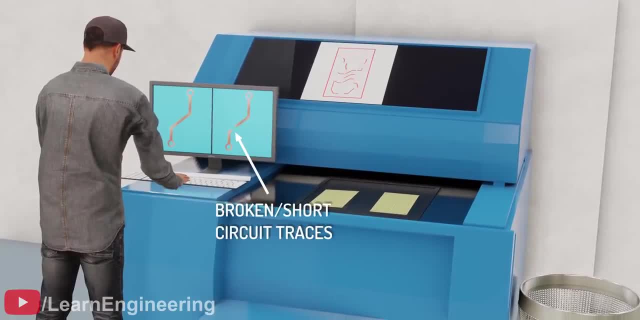 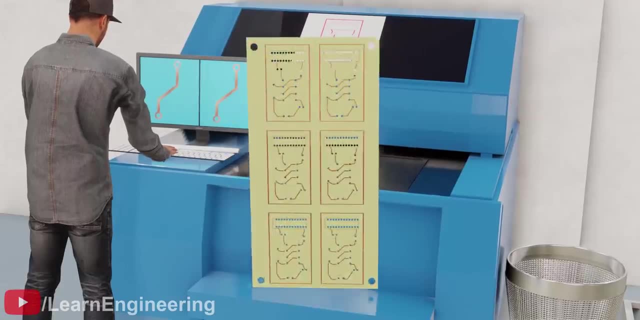 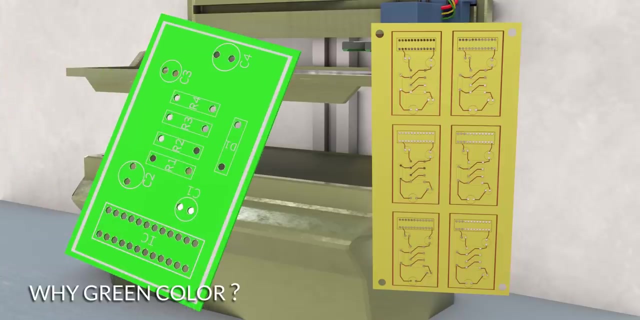 The machine checks for broken or short-circuited traces, and the PCBs with damaged, short-circuited traces are rejected. If everything is good, then boards are moved to the next step. Have you ever wondered why a PCB is always green? 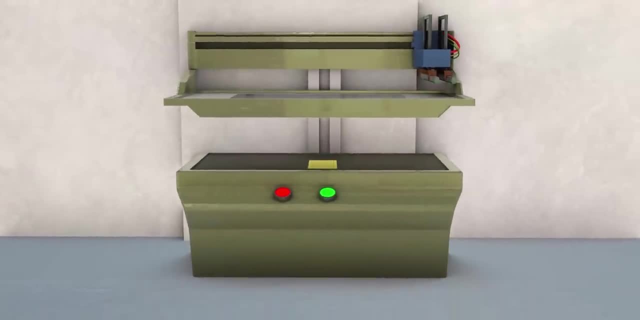 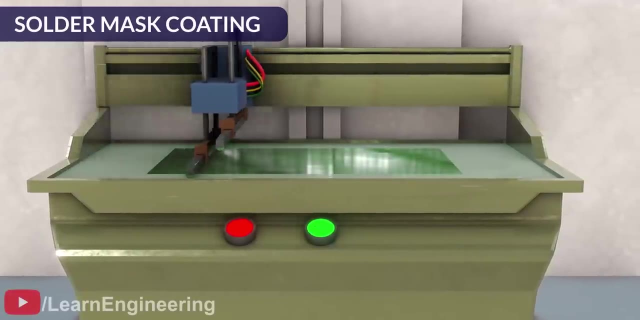 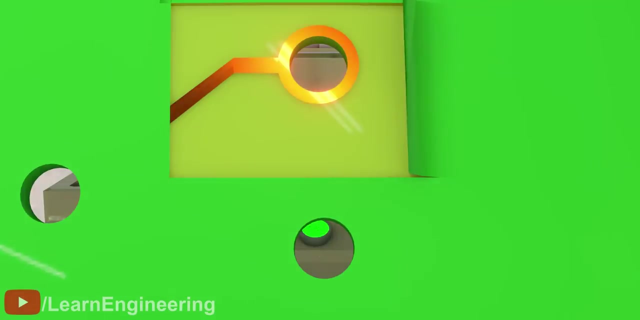 This is to protect the board from oxidation and exposure to dust. A layer of solder, mask resin protective coating is applied over the board. This layer gives the board its green hue, which has simply been universally adopted. The copper traces go hidden beneath the green layer after this operation.